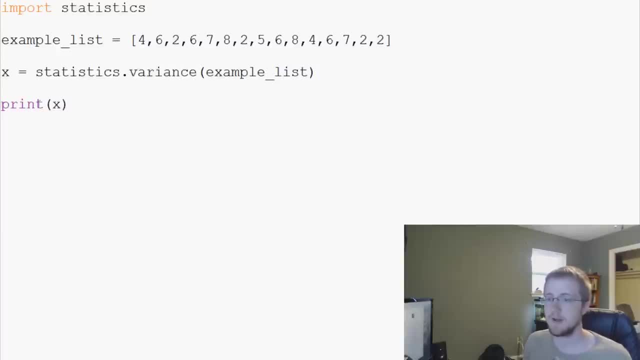 Exactly what you want, I guess. So with that, let's go ahead and get started. So we're going to go ahead and I guess we can get rid of this, And so you've seen, for now, import statistics, And so the idea here is we import statistics and then we can use this module. Now, a module is just a Python script for the most part. Some modules are a little more in depth, but this is a Python script And so I can even show you guys this: We can go to your computer: see Python 3.4 lib. 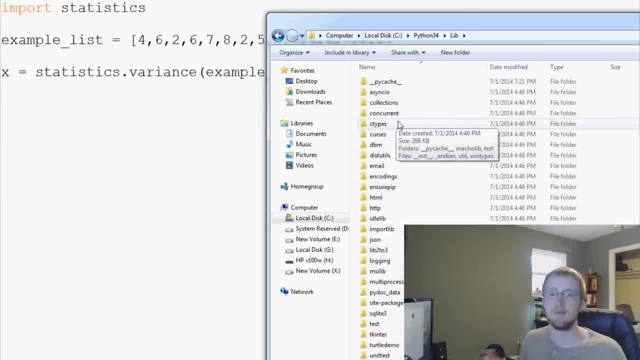 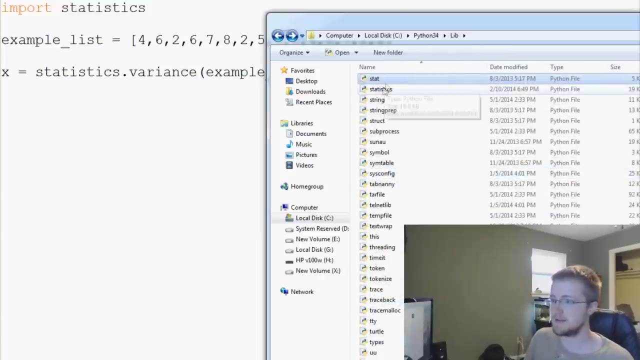 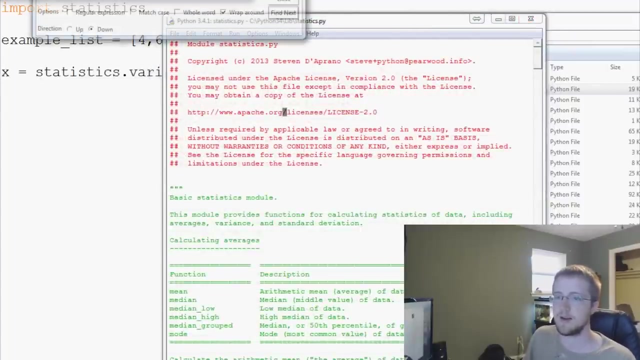 And within lib is where you're going to find all of your kind of like vanilla modules, the ones that come with Python, And then all your third party modules generally are going to be installed under site packages. So these are all your third party modules. Now statistics comes with it, So we can actually just find statistics and we can find, say, for example, the mean module We can search. Let me bring it down here: Search for like, define, mean, like that. And here is our mean function. 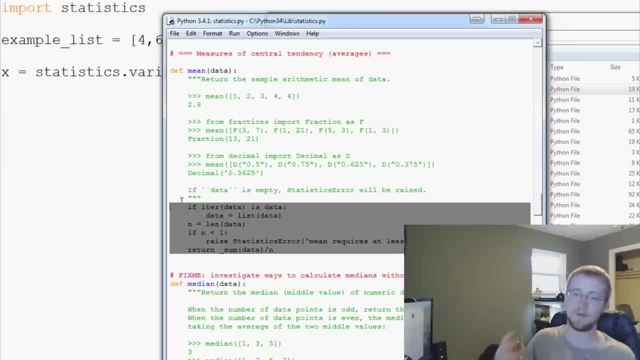 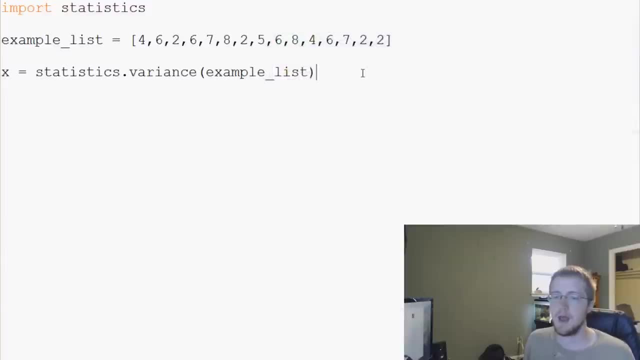 So this is the block of code that is run when we reference mean OK. so that's all it is. It's just a Python script. So we'll get out of here, minimize this And now we can go over some things. So statistics, while not super long, it's kind of a long name. We might. maybe we don't want to type out statistics every single time. It's kind of a tedious thing to type out. So when you do this, you can say: import statistics as S And now every time you want to reference statistics, you just have to type out statistics. 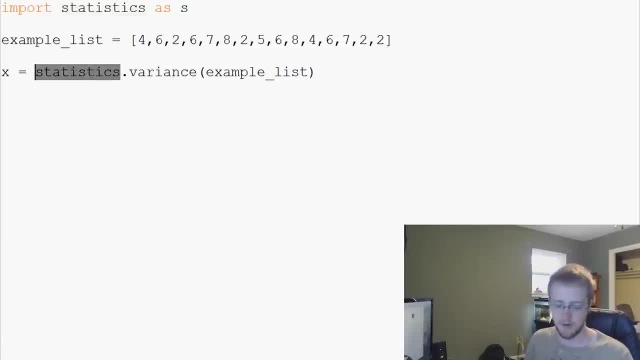 So instead of statistics dot variance, you could do S dot variance. We could run that. We didn't have it printing out, So let's go ahead and print X. And now you get your variance of 4.85.. OK, so we're able to reference it just with a simple S. Now the other thing that you can do as well is say you don't even want to type S, You just want to say variance. Well, you can do that as well, And that's going to be. 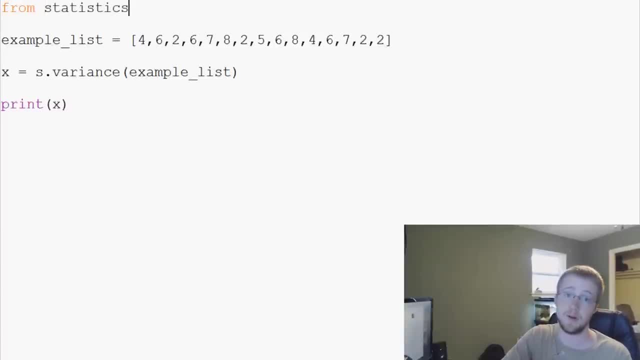 So from statistics. this is why we want to do it as S. It's a pain to type. So, from statistics, import variance, And now you don't even need an S dot. Now you could reference it straight as variance, like that. OK, so you can do that. So now, the next thing that we can do, of course, though, is from statistics, import variance. If you don't want to type variance, you could say import variance as V, Right, So now, instead of variance, we can just say X equals V. example list: Run that. 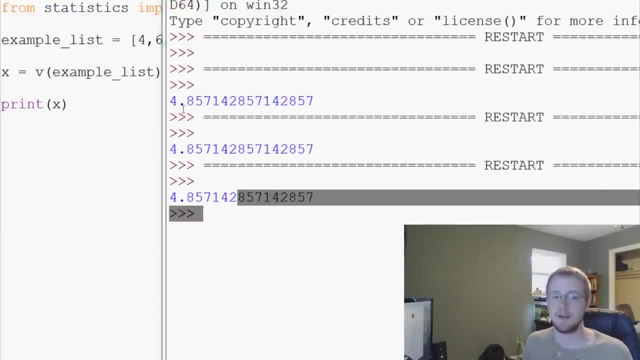 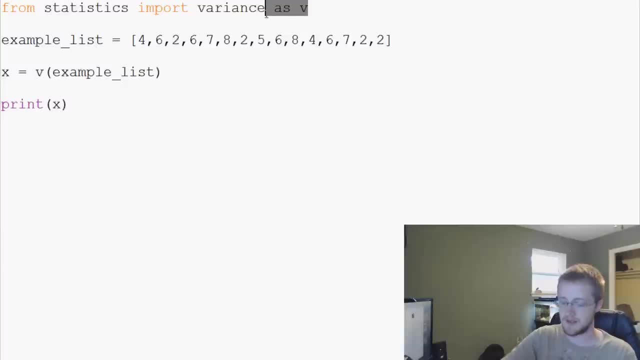 And again, that still works. Now the next thing that we want to do, like, let's say, we want to import a few things from statistics, So variance, and we want mean, So X equals variance example list, Y equals mean example list, And then we'll have it print Y And so here under this, we can see that we were able to use these commas. 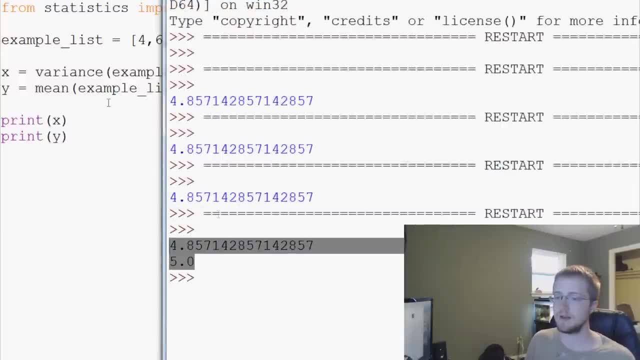 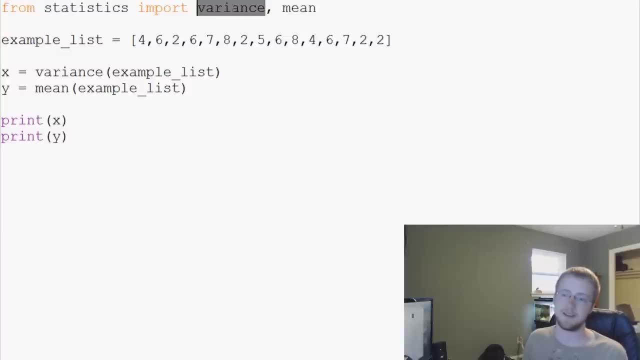 Right. So when we go and run it, we've. we were successful in pulling out the two functions from this module and leaving the rest, And then we're also referencing them as you know the function name, because we can just import statistics and the new statistics dot, And we, when we import statistics, we've imported everything anyways. 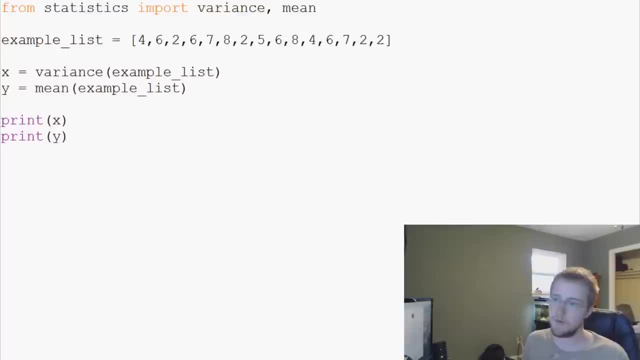 So, but we still what? if we don't want to type variance and mean, well, we can do still like this, import variance as V, mean as M, So we can change this to V, change this to M, And everything works as we hope. So we're able to do that. Now the last thing I want to cover is what, if you know we want to import everything from statistics but we don't want to have to put statistics dot, Well, we can do something else. We can say: from statistics, import asterisk, And what the asterisk means is everything. It's for regular expression. that just means everything. 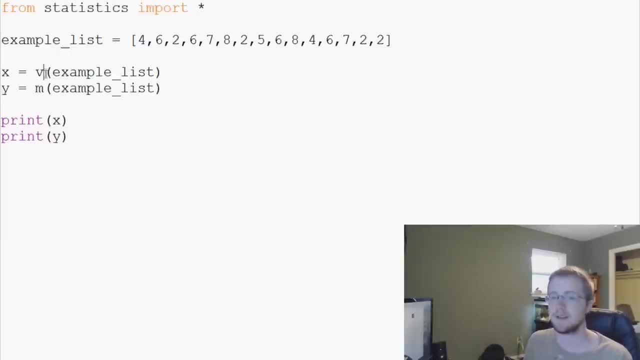 So basically we're importing everything as if we had typed everything out. so now we can say: variance mean like this: we never actually imported them, but we, we said, import everything. and then in this scenario we don't actually have to type statistics either, so we can do this and